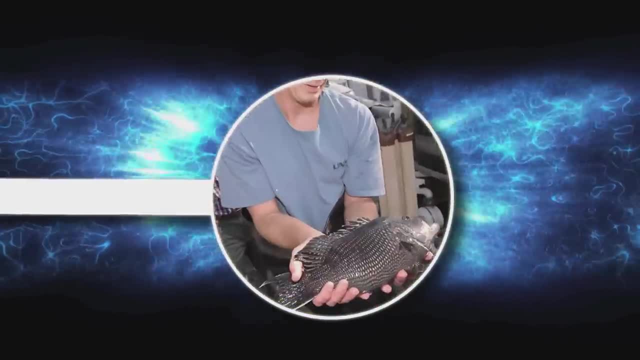 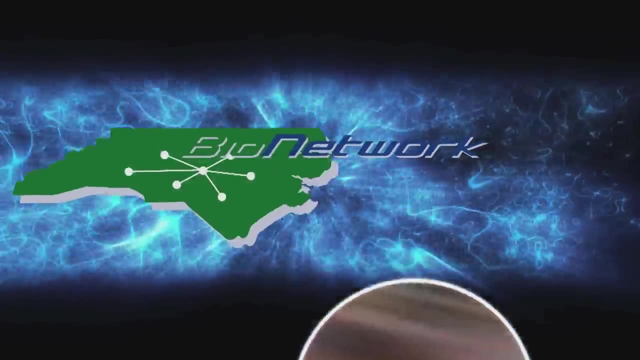 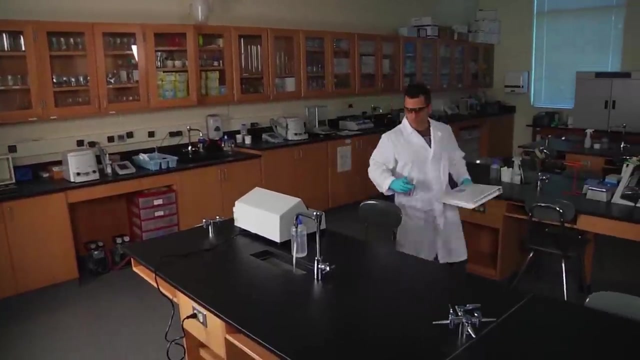 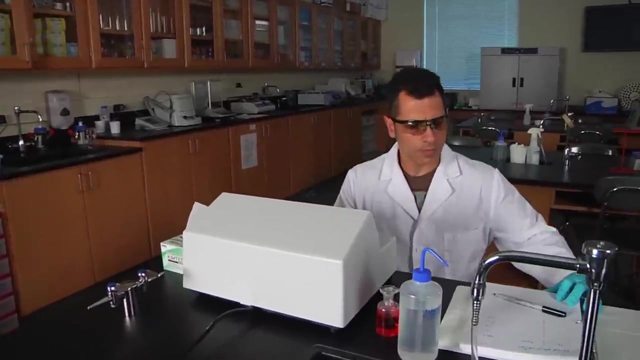 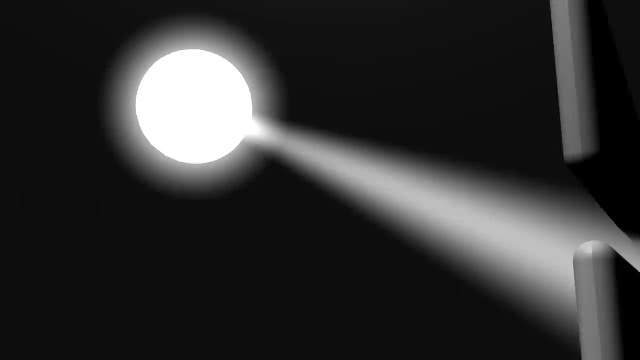 The spectrophotometer is an instrument used to measure the effect of a sample on a beam of light. We can learn a lot about a substance by studying the way it interacts with light. Here's how a spectrophotometer works. A lamp provides the source of light, The beam. 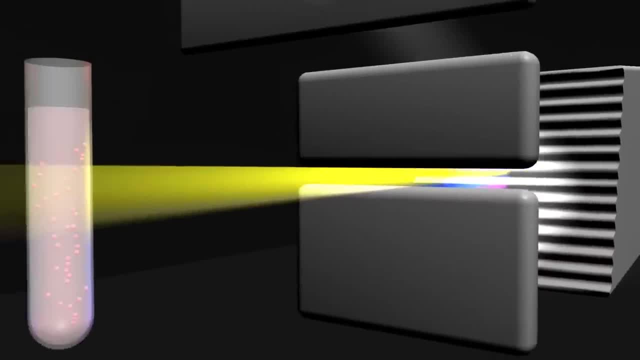 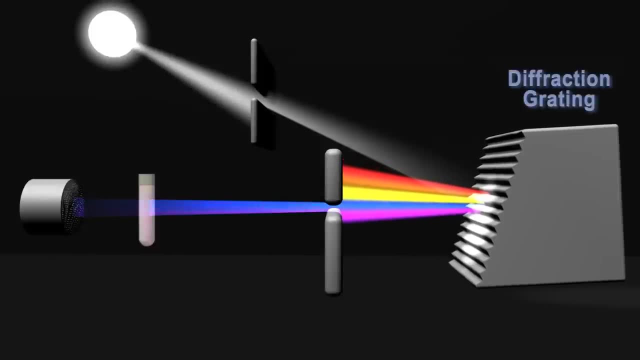 of light strikes the diffraction grating, which works like a prism and separates the light into its component wavelengths. The grating is rotated so that only a specific wavelength of light reaches the exit slit. Then the light interacts with the sample. From this point the detector measures the transmittance and absorbance of the sample. 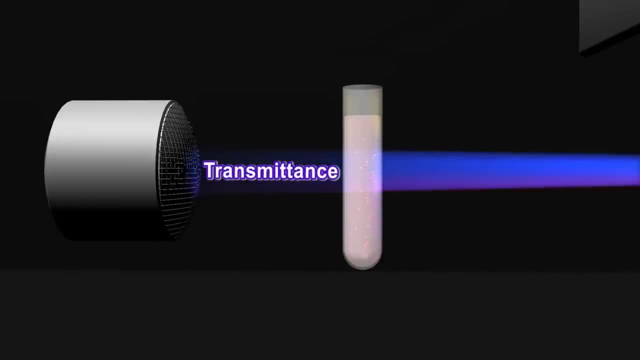 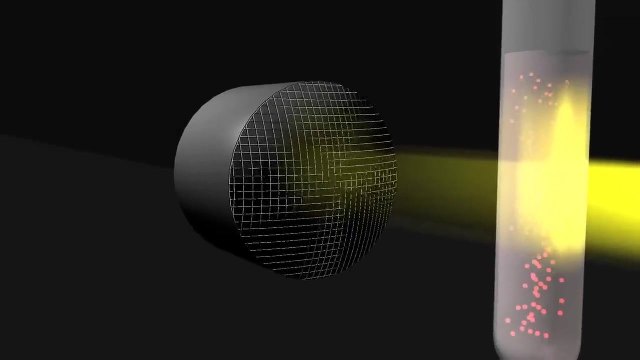 Transmittance refers to the amount of light that passes completely through the sample and strikes the detector. Absorbance is a measurement of light that is absorbed by the sample. The detector senses the light being transmitted through the sample and converts this information into a digital display. Let's practice by performing a simple experiment. 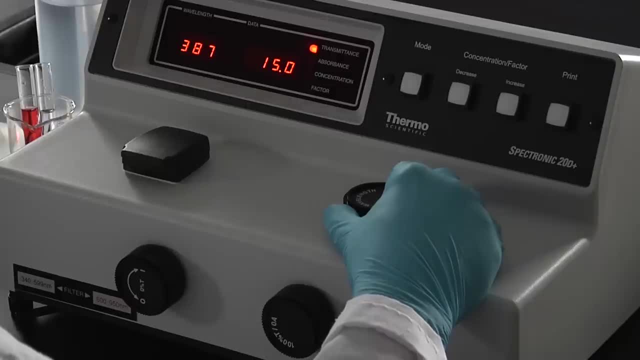 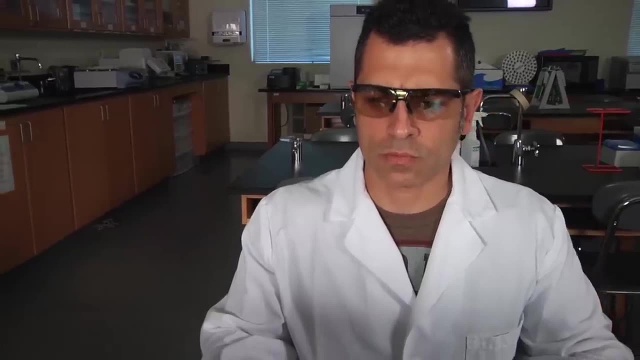 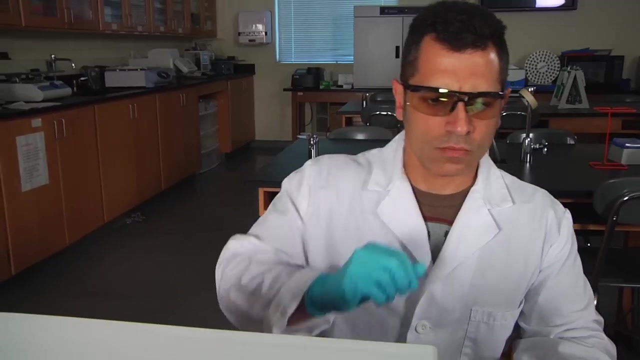 In this exercise, we'll determine the absorbance spectrum of red food coloring. To begin, set the wavelength to 380 nanometers, With the sample chamber empty and the lid closed. set the display to 0% transmittance by using the zero control knob. There are 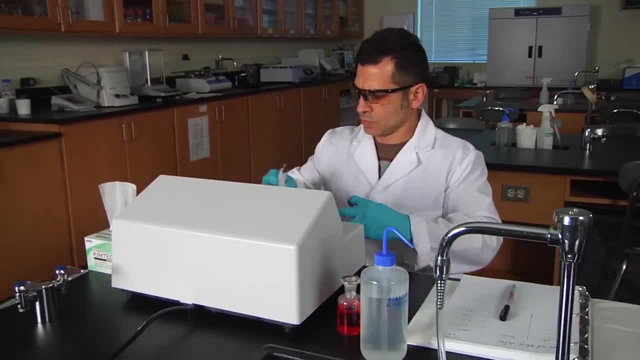 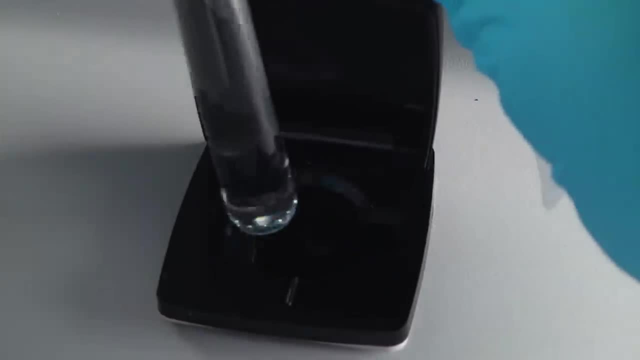 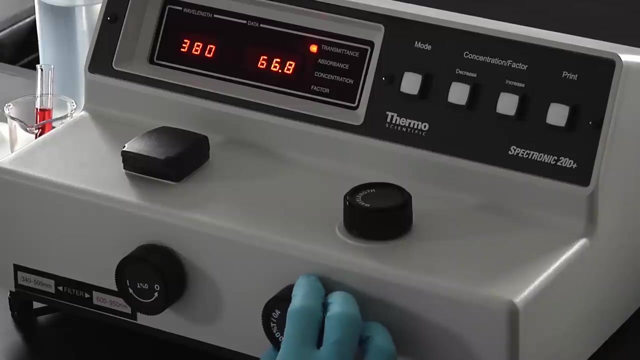 two cuvettes. One contains only milli-cu water. This is our blank Wipe, the blank cuvette with a kimwipe to remove any fingerprints and place the cuvette into the sample chamber. by aligning the guide marks, Adjust the display to 100% transmittance. 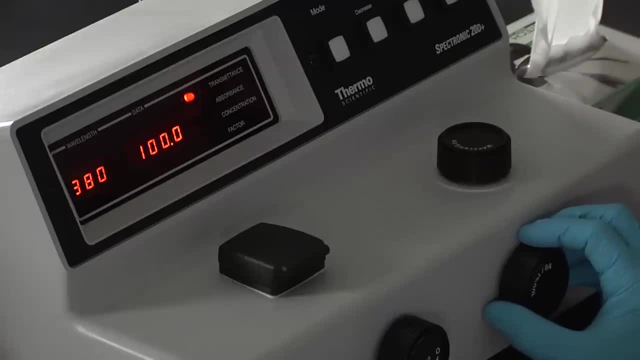 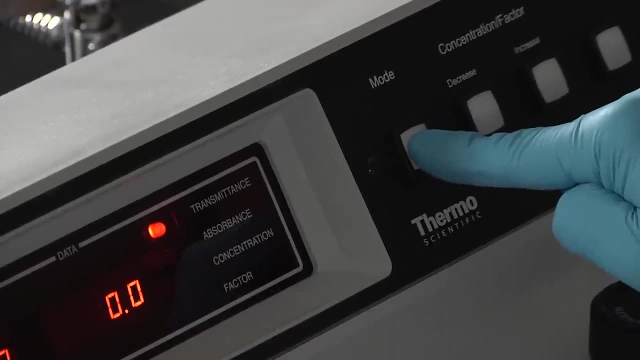 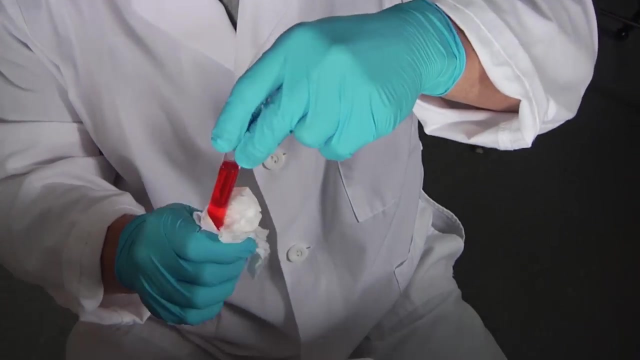 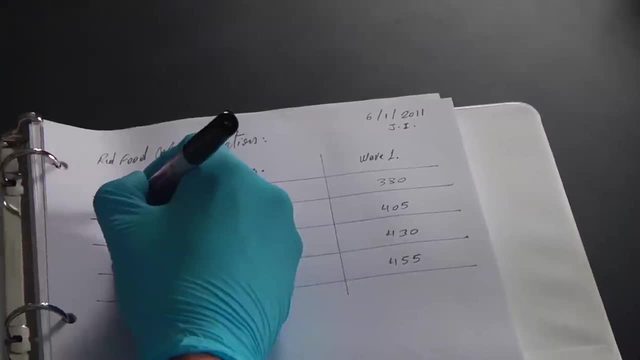 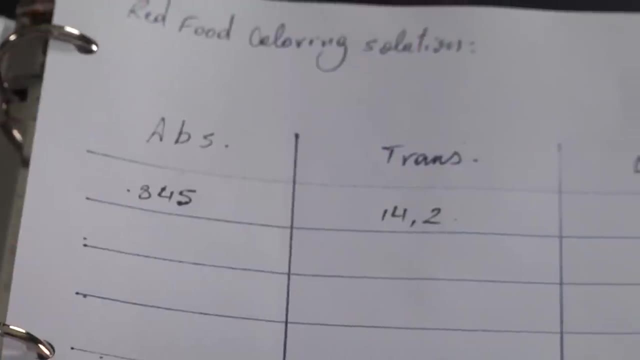 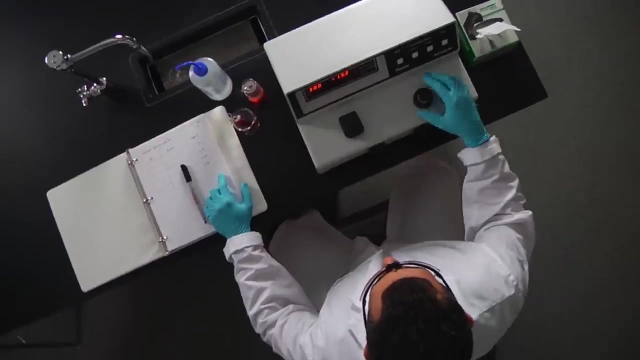 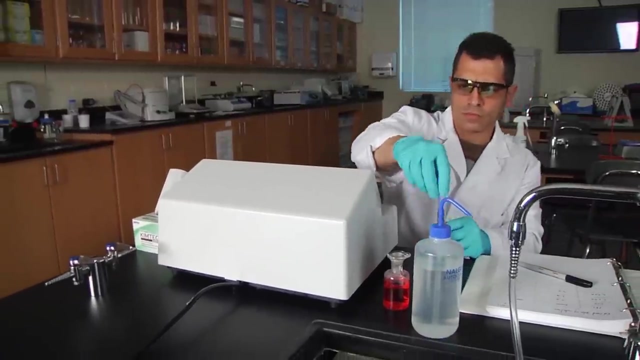 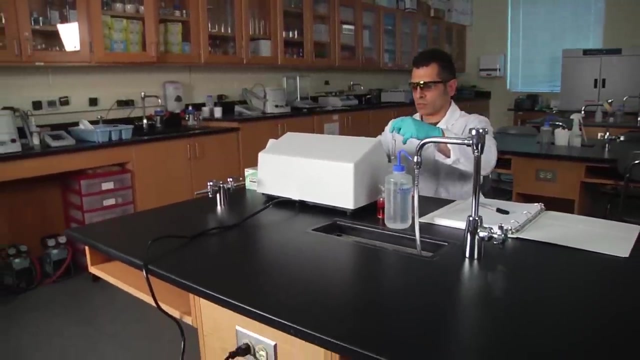 This is our sample is 0.845.. Press the mode control key to select transmittance. The transmittance for the sample is 14.2 percent. Increase the wavelength by 25 nanometers to 405.. Wipe the blank cuvette again and place it in the sample chamber. Adjust the. 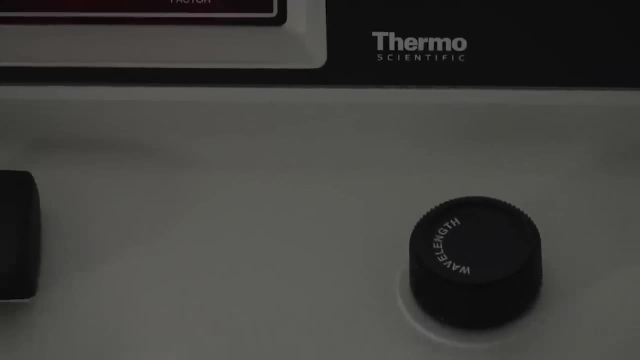 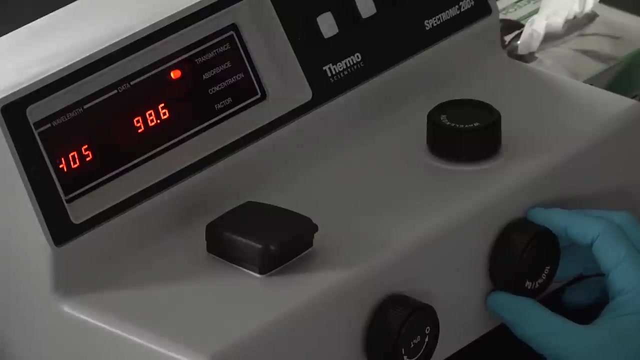 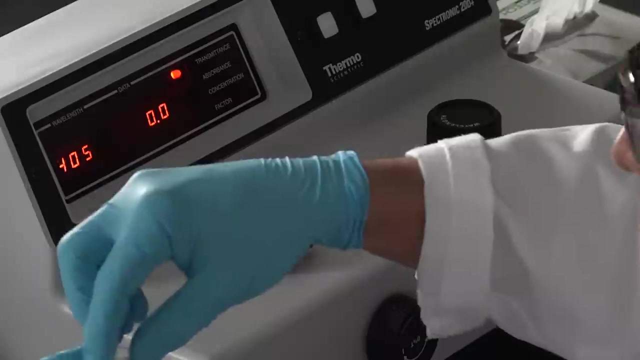 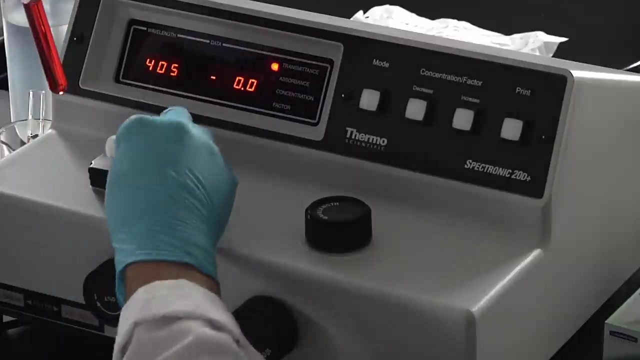 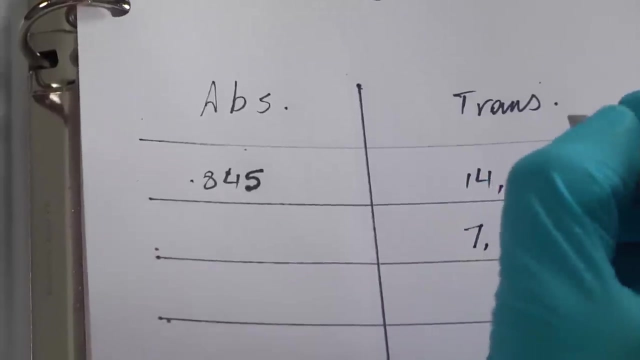 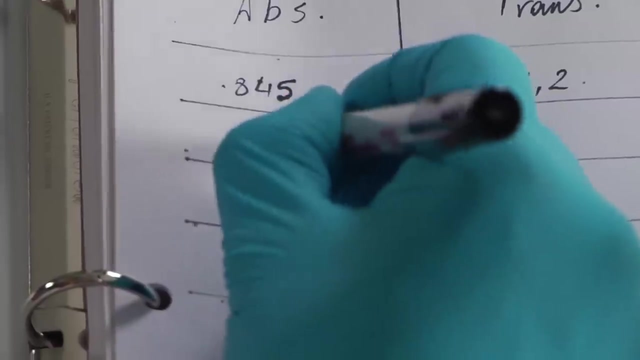 transmittance control knob until it displays 100 percent. Now remove the blank, Wipe the sample cuvette and place it in the sample chamber. The transmittance for the sample at 405 nanometers is 7.4 percent. The absorbance for the sample is 1.130.. Record. 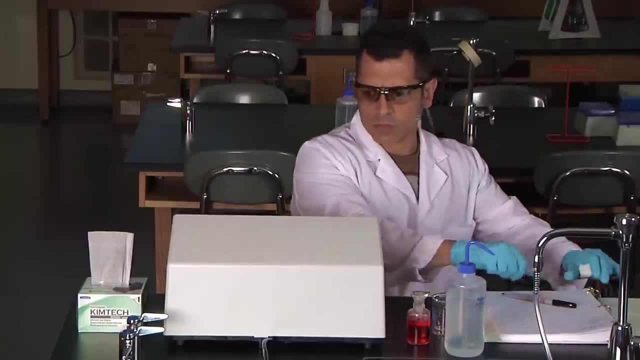 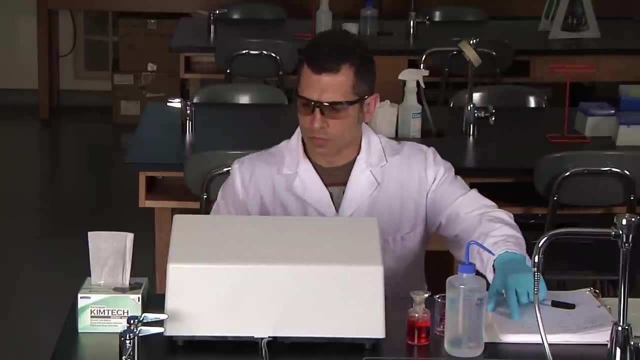 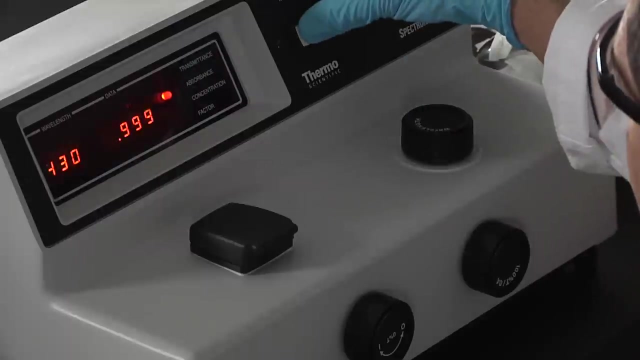 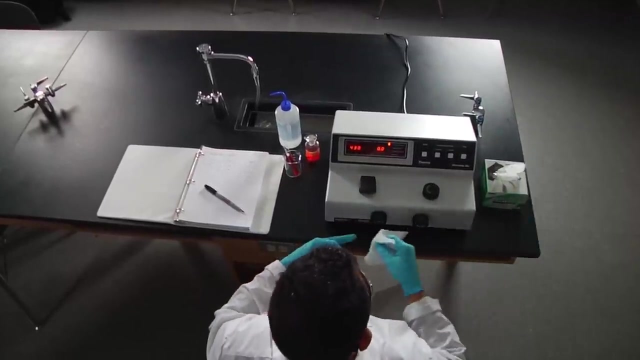 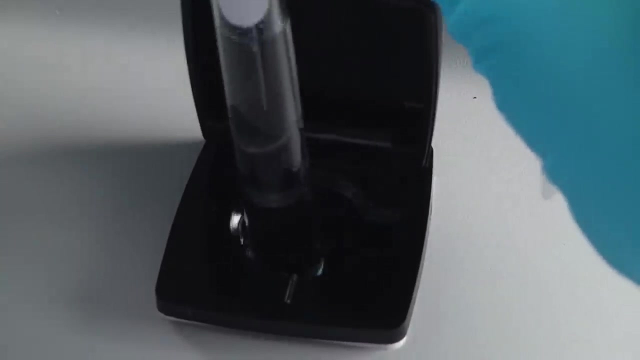 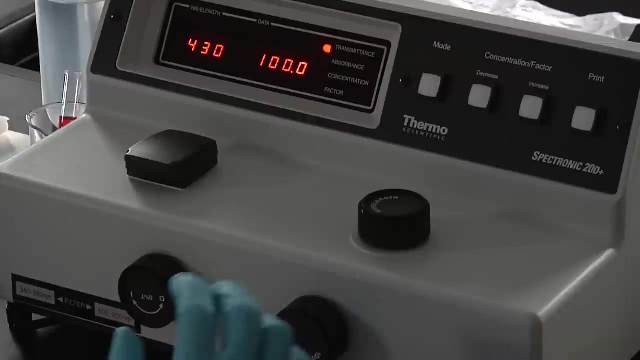 this in your lab notebook. Increase the wavelength by 25 nanometers to 430.. Repeat these steps with the blank and sample writing each value in your lab notebook. Theチェine given to the sample, bİ esté here, indicates the actual wonders of theinization. 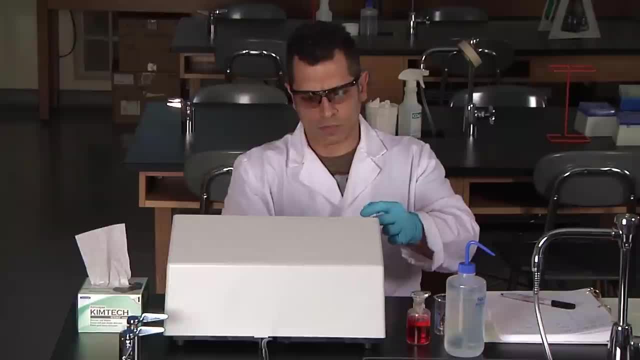 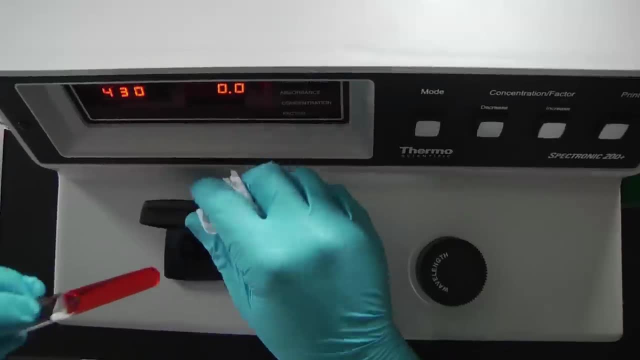 Did you notice any change? Racem stand at the right altitude. The nota: if positive Southern is taken in the current threshold and the indiciaton is taken away, The dot value for strawberry is jego radian, which we can solve in various showcases. 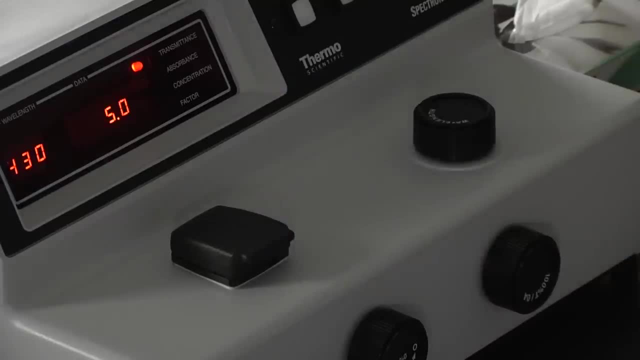 Point, Chloridite, Quantitimum and interval. For example, if rate is positive, the always change. Readор lagiер and rarikari study powerd 베i ar, presented Non Lyon Ichthrough, guys cárre liêr, veõk brýnders.